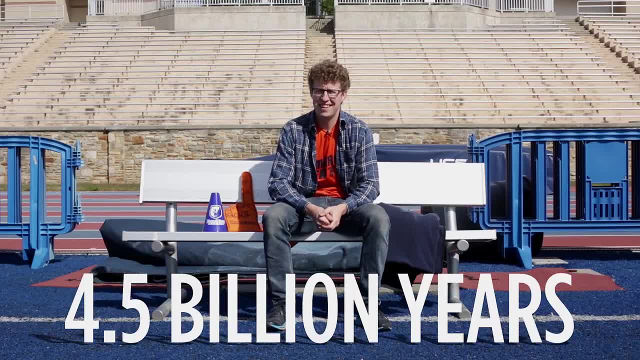 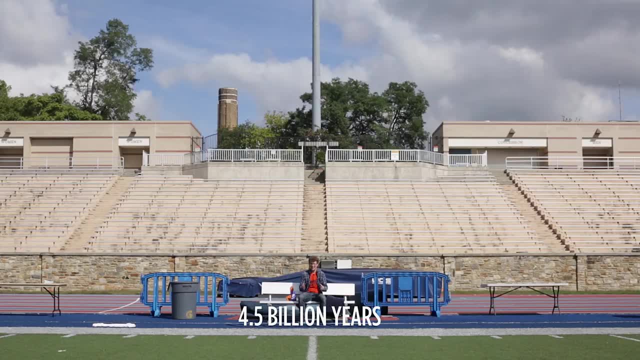 How can you imagine 4.5 billion years? And how does that compare to the amount of time that humans have been around? A geologist gave us the idea to use a football field as a metaphor, and that's exactly what we're going to do. 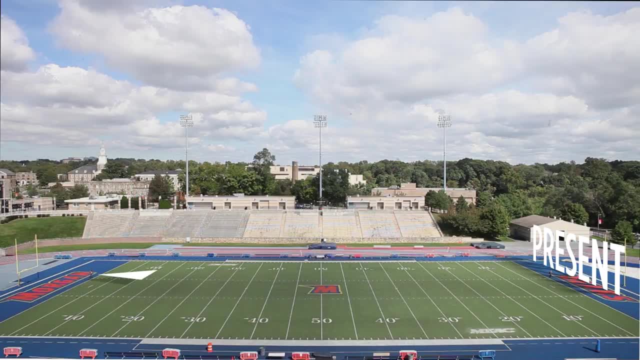 At this end zone, we've got the present. And at this end zone is the moment our planet formed. 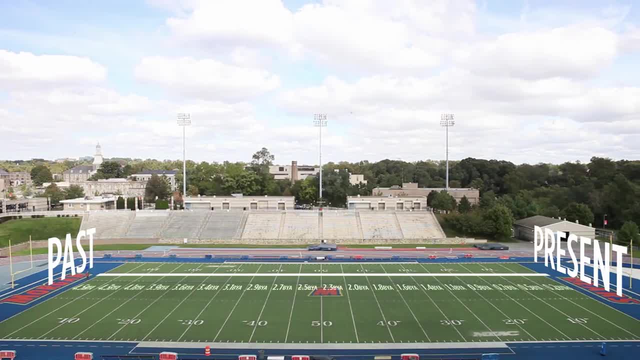 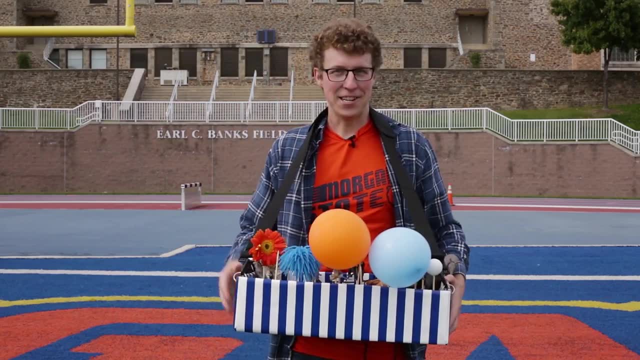 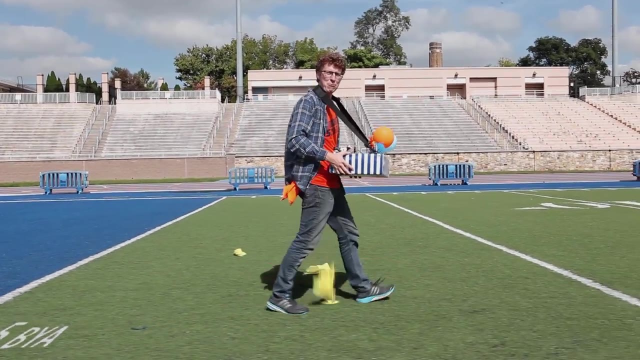 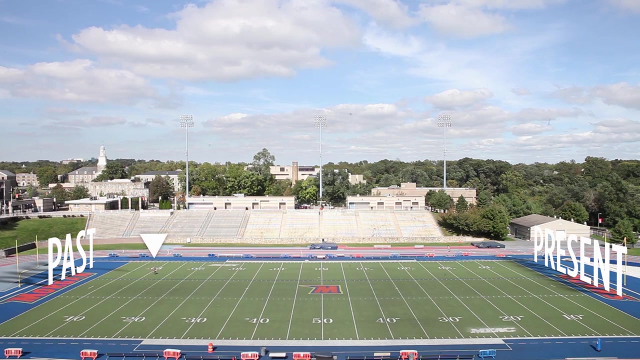 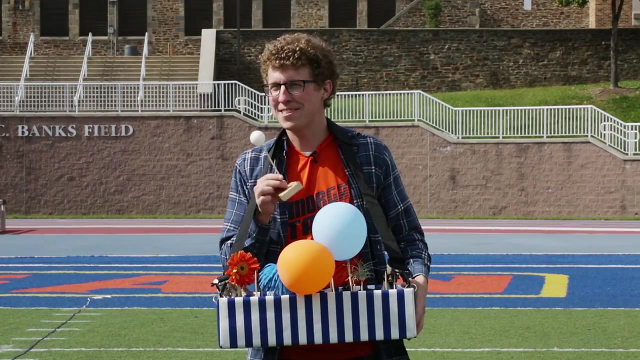 Earth's entire history stretches the full hundred yards in between. Every inch is 1.3 million years. Let's start at the beginning and take a walk through Earth's entire history. For the first few hundred million years, the Earth was bombarded by rocks from outer space. But now it's starting to calm down, and way up here 3.8 billion years ago, life begins. We're talking simple life. Single cells floating in a vast ocean. 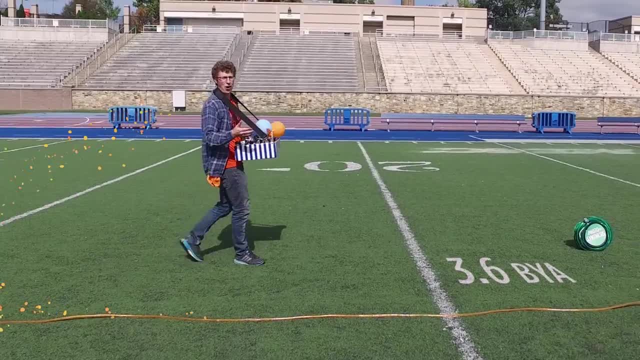 Now these cells are figuring out new ways to get energy. They're evolving to harness the power of the sun. 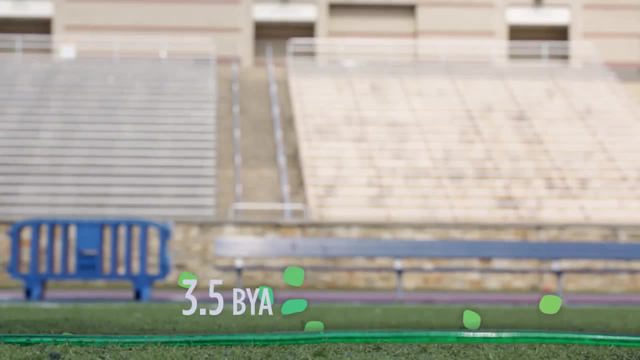 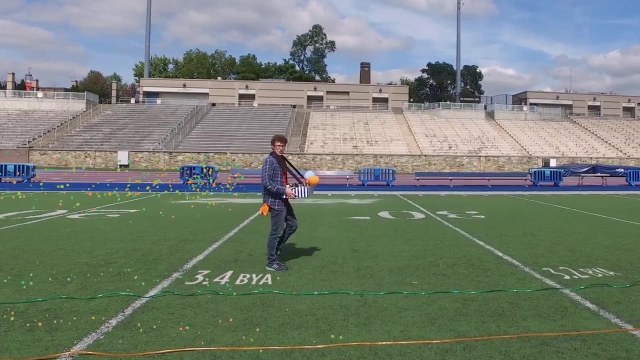 Photosynthesis starts past the 20-yard line. The air here is mostly carbon dioxide and nitrogen. But right around here, little green cells start making oxygen. 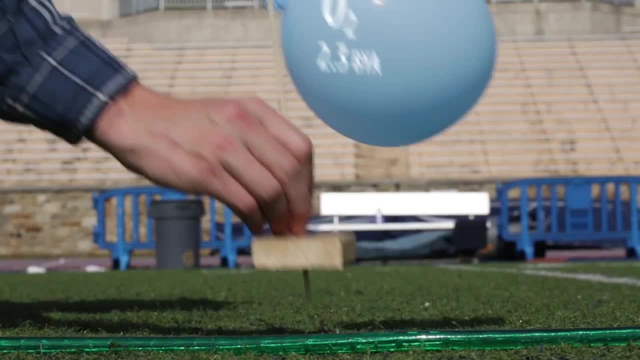 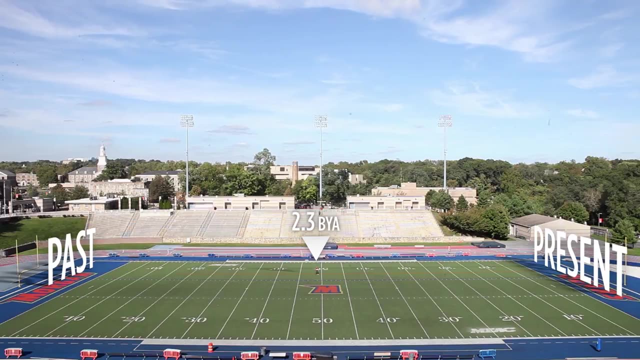 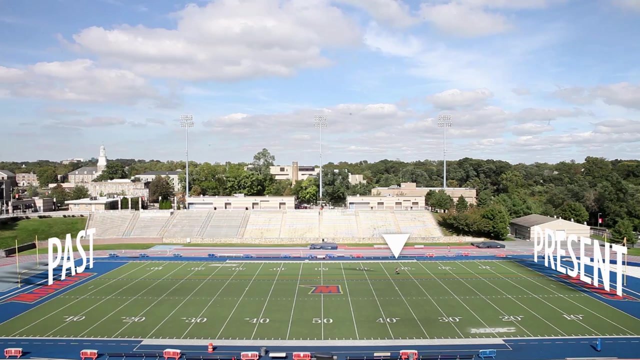 And up here, about 2.3 billion years ago, oxygen starts building up in the atmosphere. We're halfway down the field, and we just got the kind of atmosphere that humans can breathe. For the next billion and a half years, it's paradise for single cells of every variety. 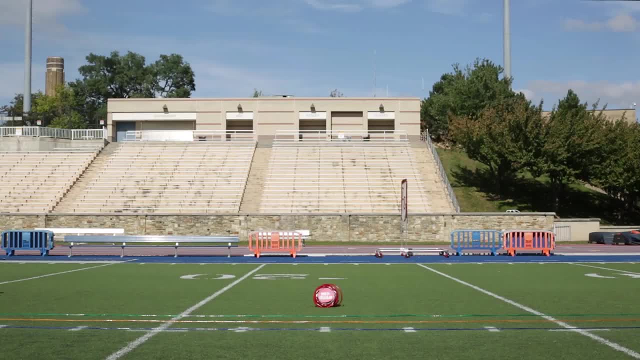 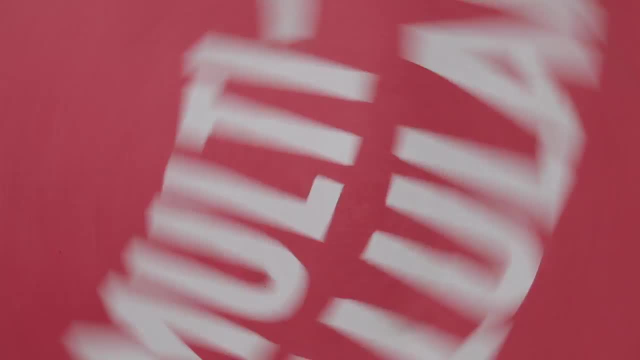 But as we move down the field, cells start working together. And by the time we reach the 18-yard line right here, there's lots of complex critters floating around. 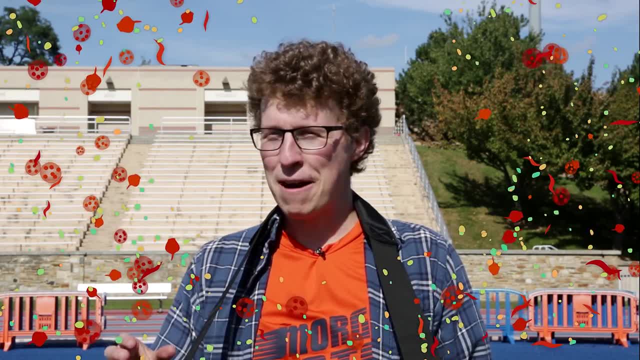 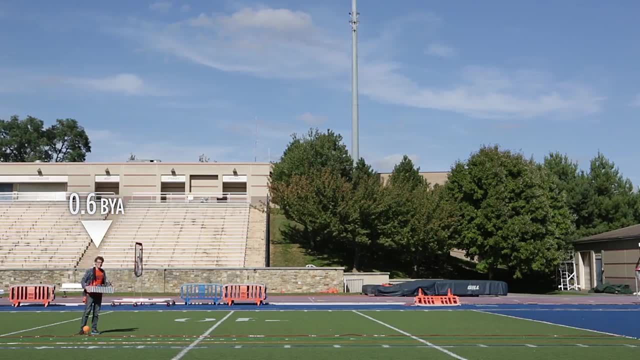 It's 800 million years before the present. And things are about to get really interesting. Here at the 13-yard line, we've got an ozone layer. And here, a sudden explosion of diversity. Fungi. Sea anemones. Mollusks. 530 million years ago, animals take their first steps on land. In the ocean, fish appear. Land plants. Insects. Sharks. Amphibians. 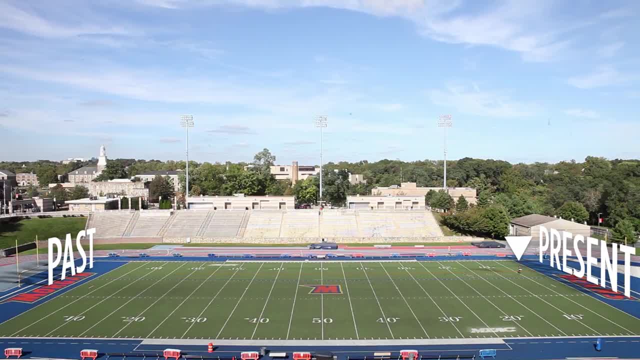 It's been 4 billion years since we started, and here at the 5-yard line, we're just starting to see the first mammals and dinosaurs. 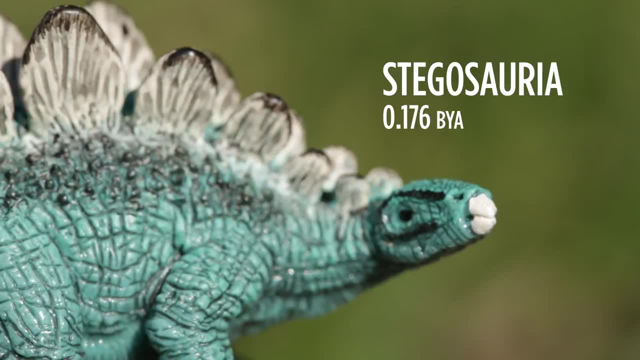 We see Stegosaurus dinosaurs right here about 176 million years ago, but we don't see the